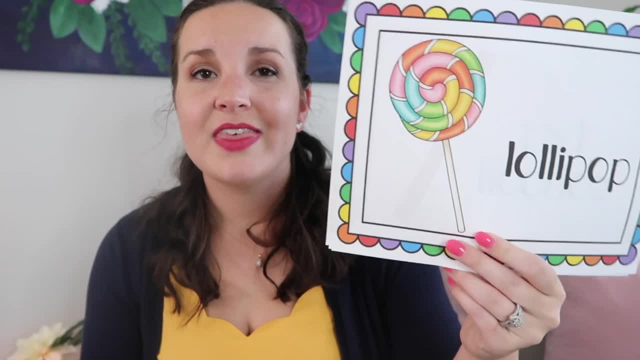 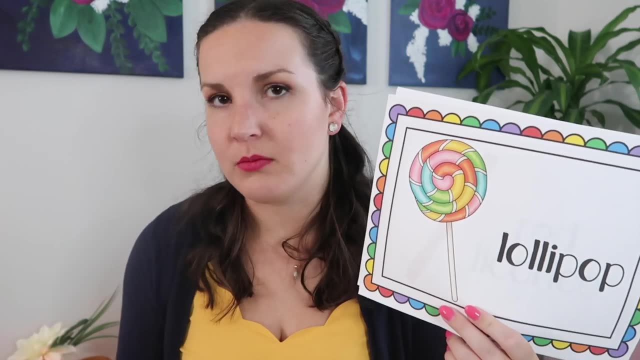 something up on the screen, or I'll pull out a card, or have a kid pull out a card that goes along with whatever our theme is And we'll read that off. So this one says lollipop, So lollipop, whoa lollipop would match ti-ti-ta. So anyone who's in the corner that says ti-ti-ta would then be out. 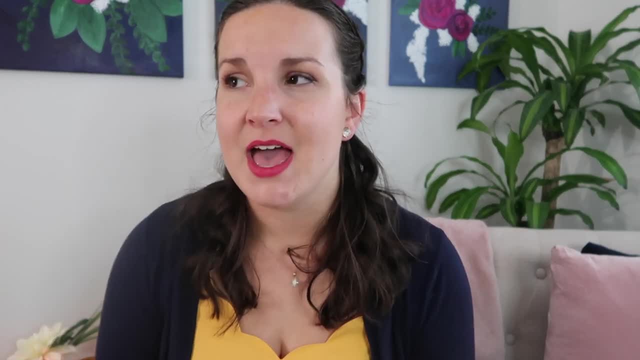 and go sit down. The reason I like to do it this way is because it makes it more random who actually gets out, And it means that we actually get out and we get out. So I'm going to do that, So I'm going to. 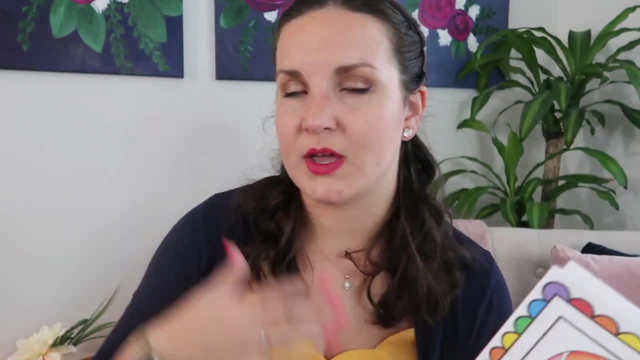 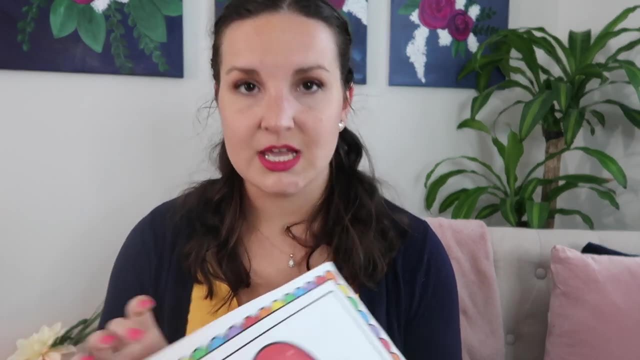 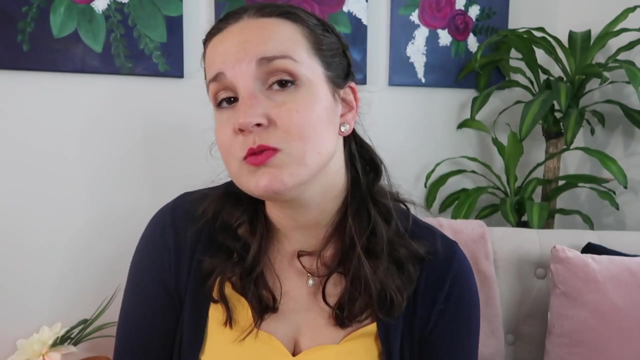 have to think about like, okay, what rhythm would this match? And we kind of talk through it as a group. So then we keep going, they count to 10, they go to another one, and then we get to the end and I pull up gumdrop: That's got two. So anyone in ti-ti would then go and sit down. You can use. 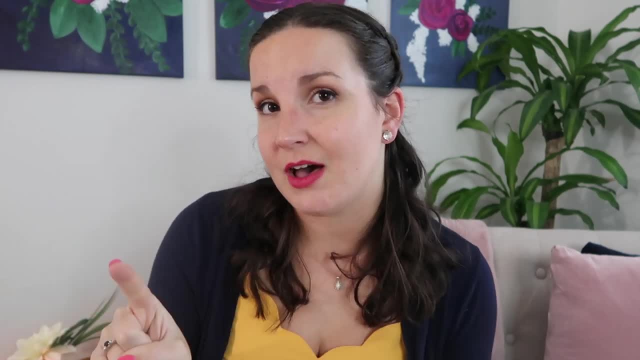 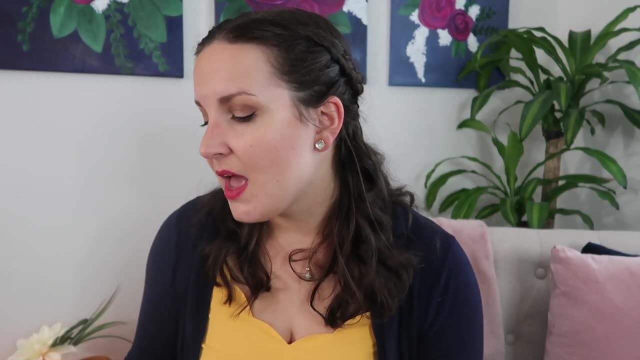 whatever rhythms you want, as long as it's like one sound. So a lot of times I'll use half note instead of quarter note, because even though it's long, it's still just one, you know, sound. So it goes with one syllable And that works really well. I also use lots of different words, So 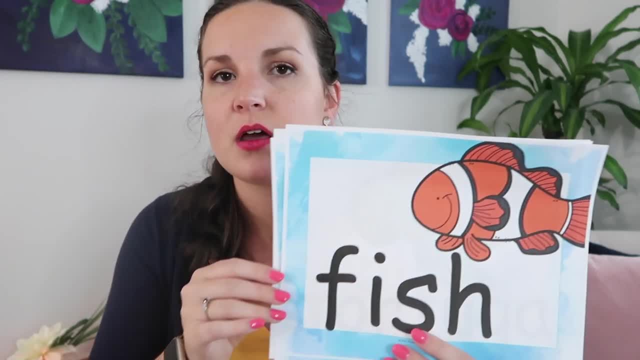 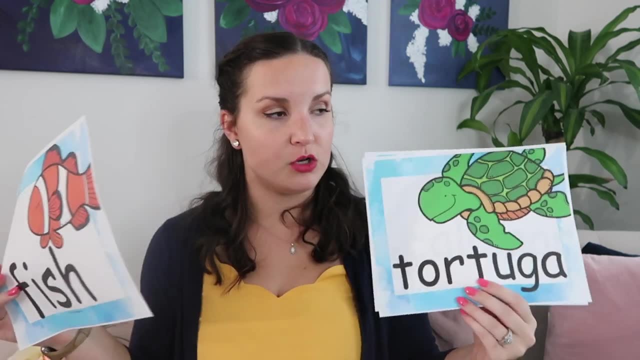 like those were all candy things. And then I also have I do like ocean animals. This one, I full disclosure: I haven't used this set yet, but I'm going to very, very soon. I'm super excited. We're going to do vamos a la mar And we're going to do this and review our rhythms because we got 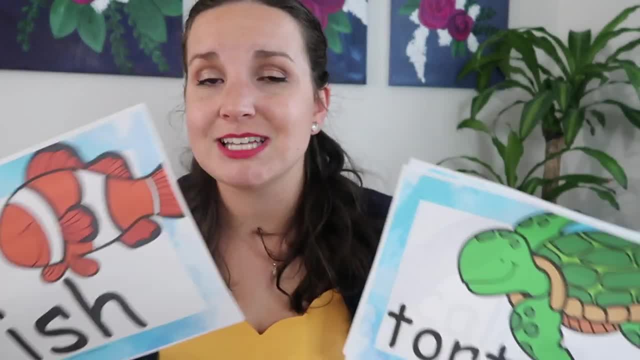 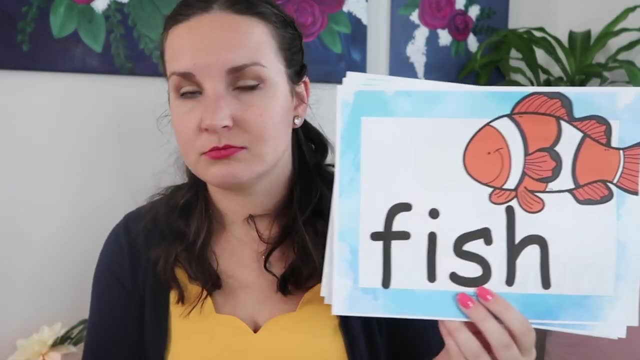 our Spanish words and our English words, and it's going to be a great time. And so same thing. tortuga would be ti-ti-ta, so those people would sit down. Fish would be ta, so those people would sit down. So that's version number one. Version number two: 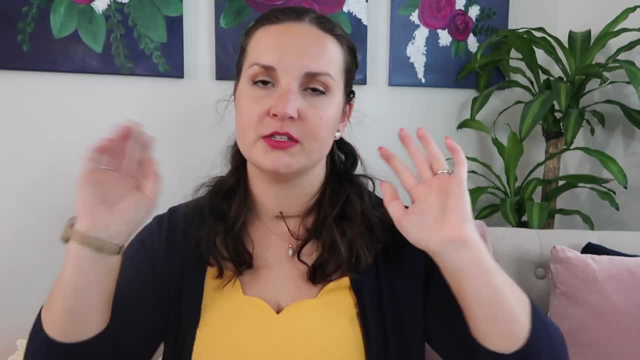 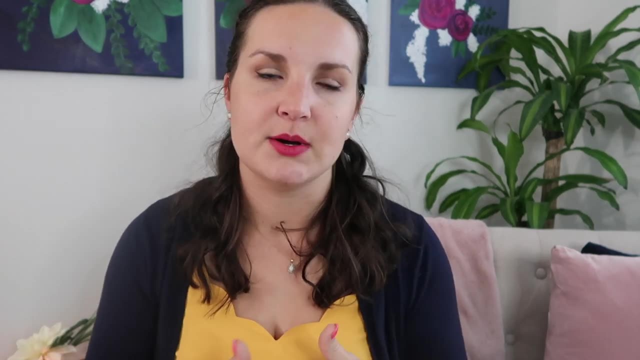 if you want to do more of an assessment is you could put the card up on the screen and then have the kids go to that corner, The downfall to this being that then kids can see where the other kids are going, And so it's not a very reliable assessment because, again, they can see where 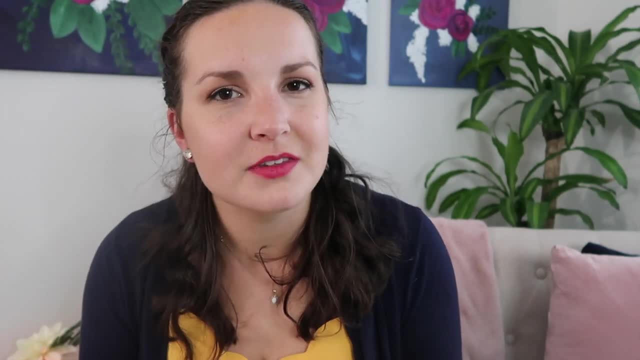 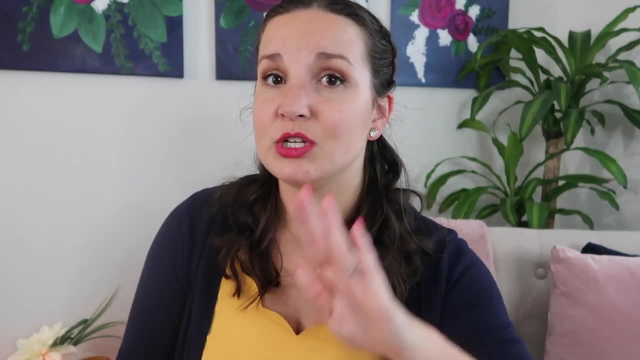 other kids are going, And so they might, you know, just go where the other people are going, which is totally understandable. If you want to make it more of an assessment, I do again, this is something you can totally make up on your own. You can draw it by hand, You can do it on. 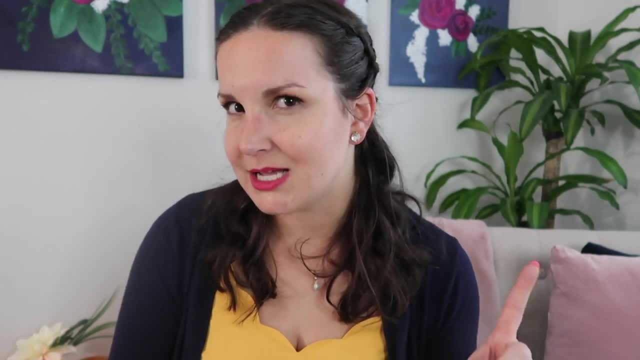 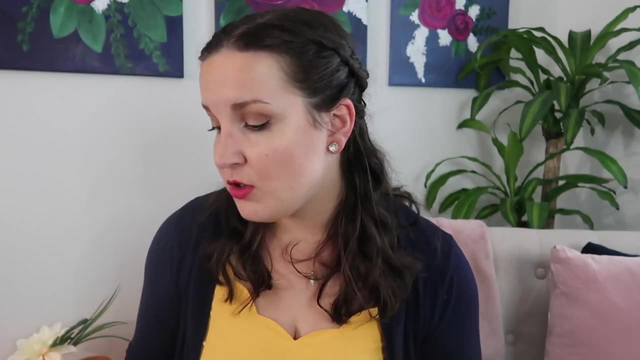 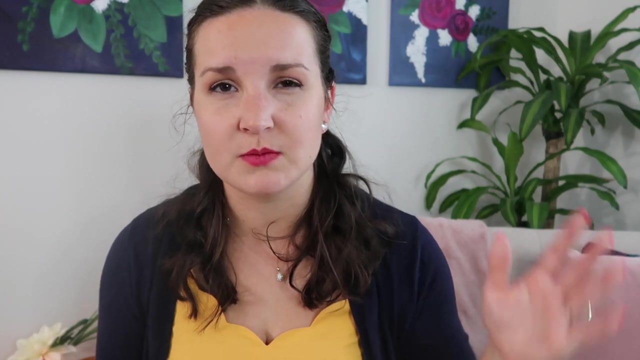 your own. So I do have these sets in my TPT shop. I will link them below And along with them you get a whole bunch of different rhythms. So you'll get half note, you'll get dotted half note, you'll get quarter note. you'll get like lots of different kinds of rhythms. So you can. 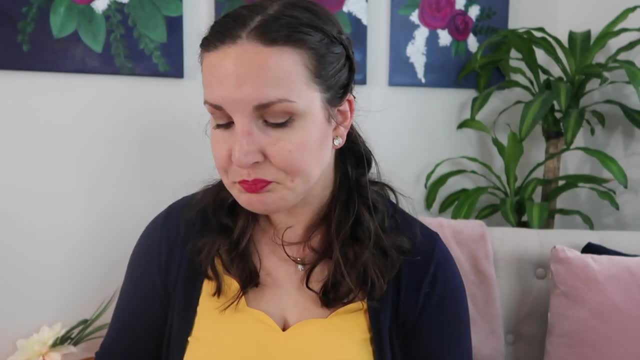 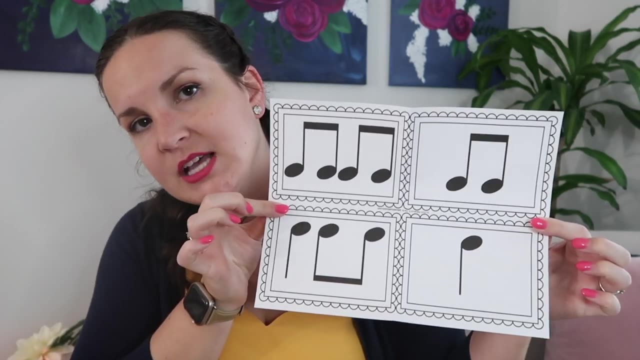 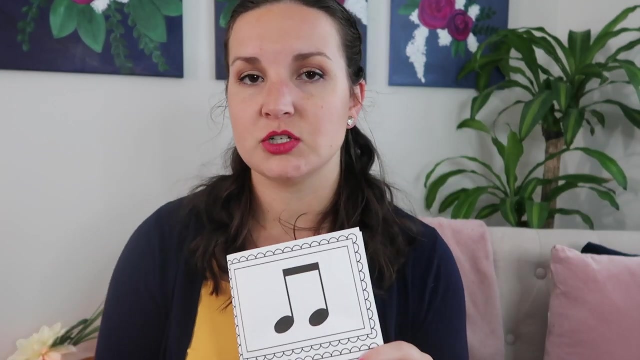 use it with all different grade levels in the one file. Yes, And then I also have two versions of assessments, So one of them is this little one, And so it has four different rhythms on it. all you do is fold it in half and then have you can put up the answers on the board and have the 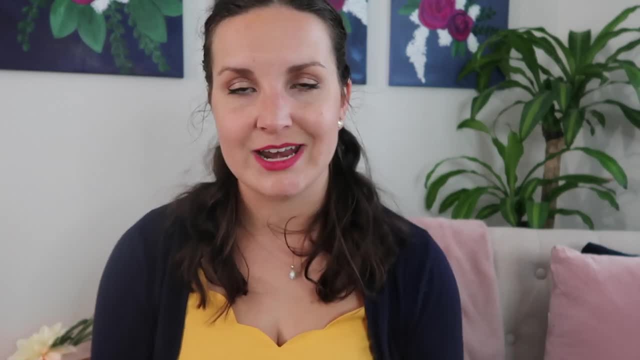 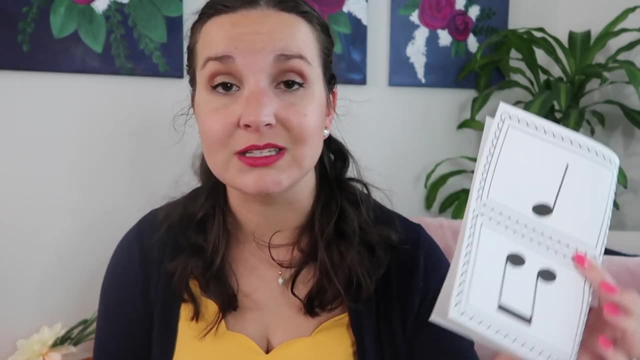 kids just show you which one it is And then you can write it down in your you know grade book, whatever you're doing to grade, And that's a super, super, super quick assessment. This would be really great at the end, Like maybe we do the active version first and then we sit down and do. 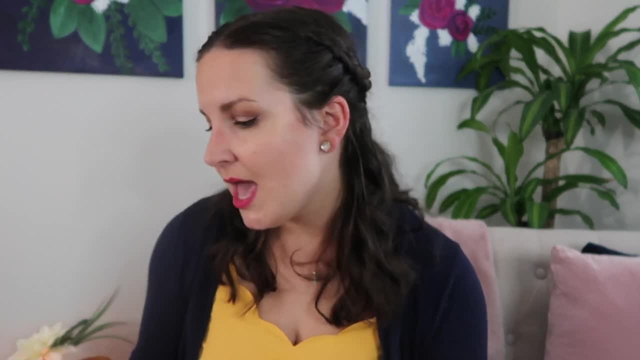 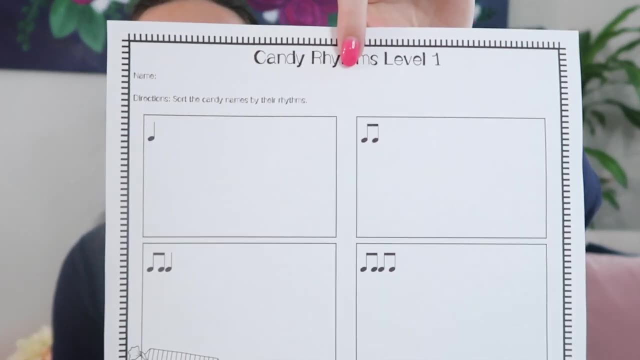 this And I take a quick assessment to see who's understanding what the heck we're doing and who has no idea what's going on. It needs a little bit more work. Then another version you can do. if you want a version that you can actually, you know, turn in. 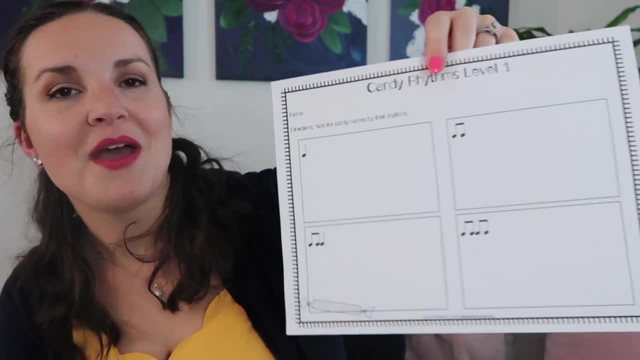 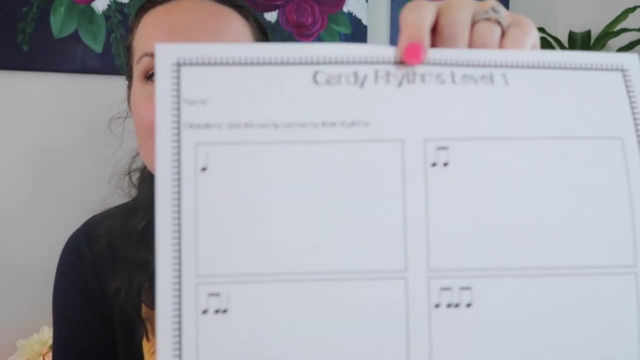 hang up on the wall. tell your administrators that you did in fact assess them is. there are also these with the four boxes, And so the kids can just write down the rhythms, or this one's candy rhythms, So after Halloween you could have them, like put pictures of candies in there. 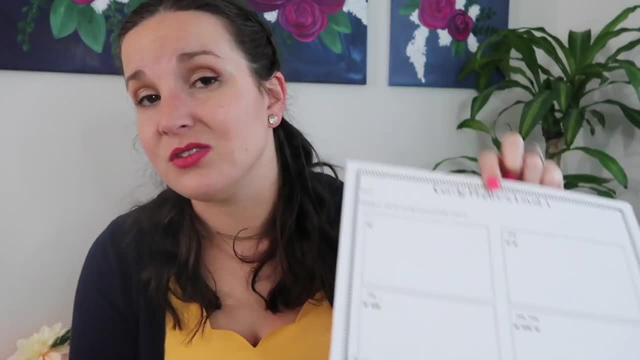 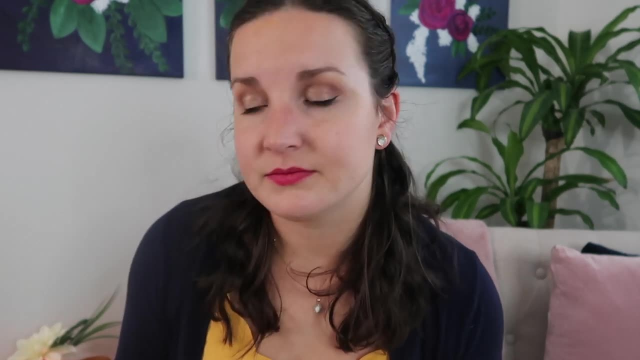 or like take their Halloween candy and like group them. Or if you're really nice, you can give them candy and group them, but your girl's not going to do that because I don't want to die. So there's that. But these two ways are really good for assessment. The other: 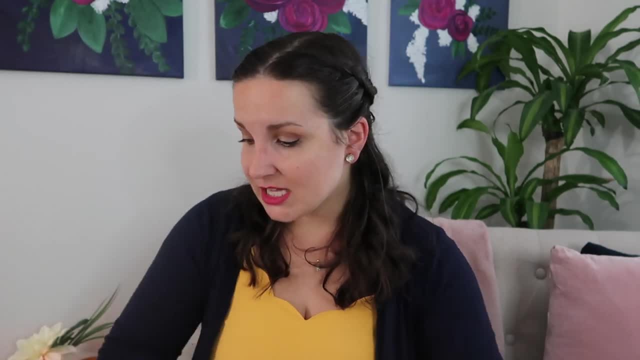 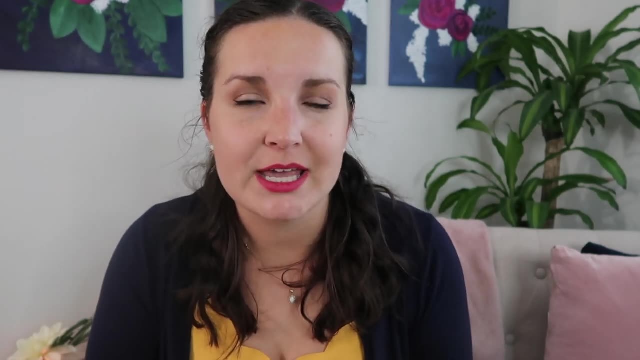 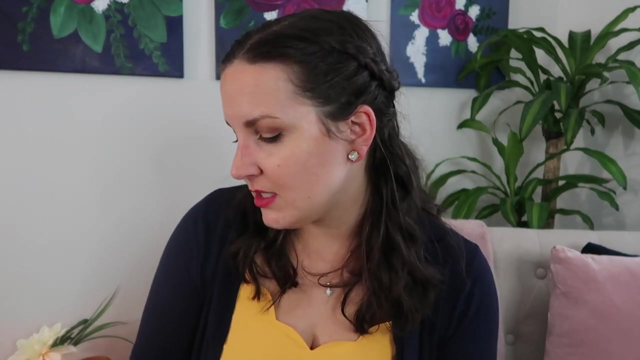 ones are more just for fun. So this has been a huge, huge hit. My kids love four corners, It is a great time, And so this is always a really good way to play it and also make it academic. You know we want to play it, but make it academic, So really really fun. I will leave these down below. 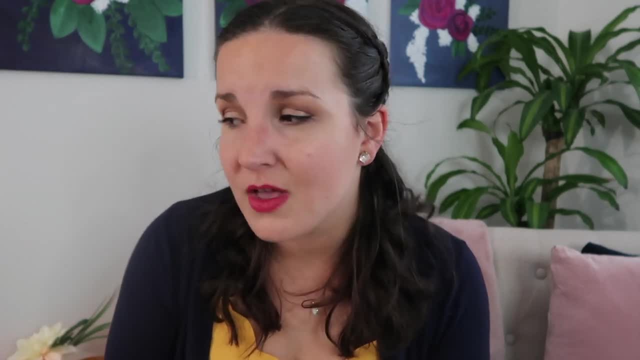 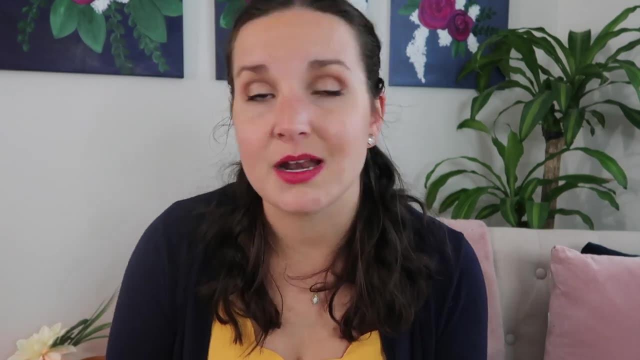 in case you want to purchase ones that are already done. but again, you can totally make it up yourself. Um, so yeah, Thank you guys so much for watching. I would love to know if you have done four corners before. If so, let me know and I will see you next time. Bye.